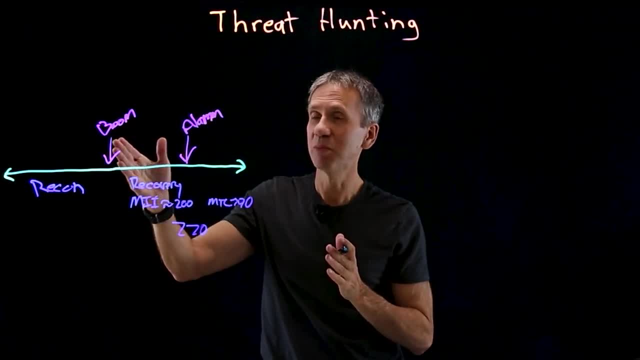 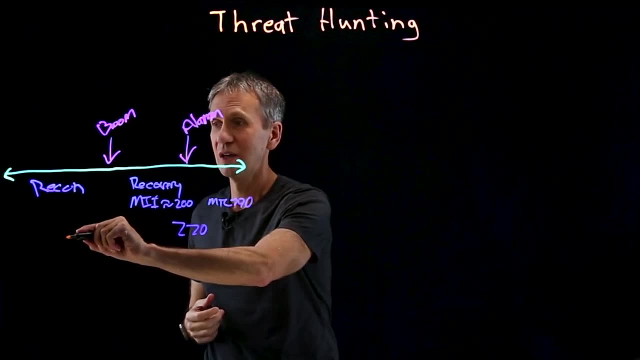 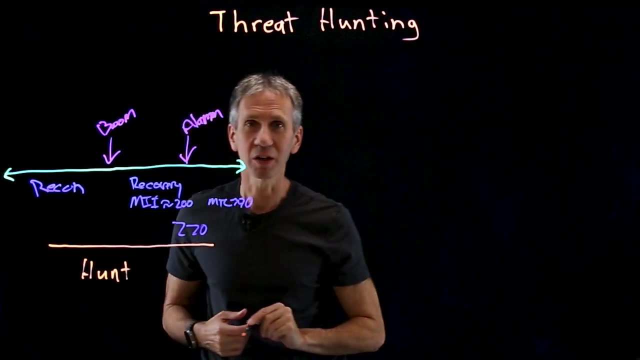 alarm and the boom closer together, or even go back before boom and start to realize during the reconnaissance phase that something is amiss, something is happening. in this phase And this timeline in this area is when we could be doing what we call threat hunting. I could do a hunt. 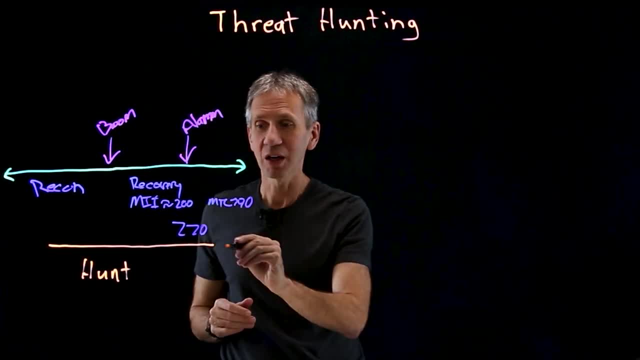 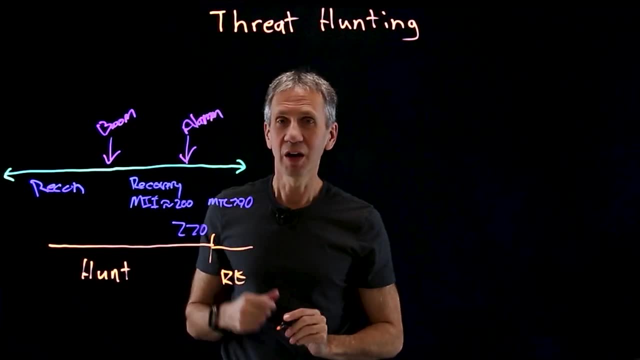 and we'll talk about what that involves After the hunt. it's when we start doing the investigation, And the investigation is reactive. The hunt is proactive. That's the big difference here. So, as much as possible, it would be nice if we could go- 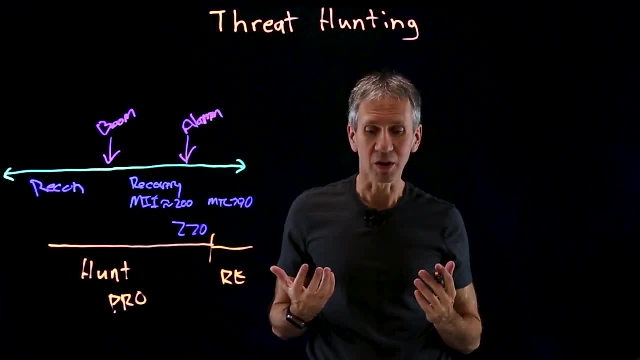 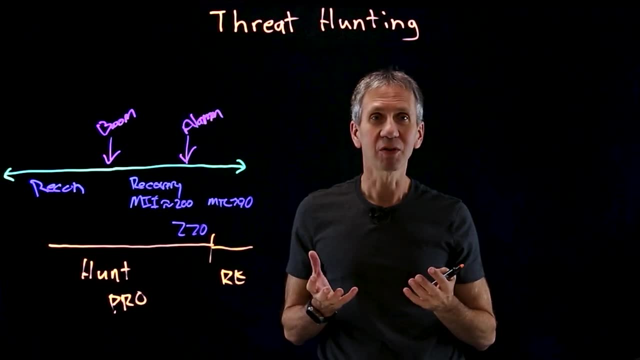 back and anticipate some of these things. Now, how does this work? Well, it turns out we're going to take- if we're doing threat hunting, we're basically going to develop a hypothesis: You have someone that's acting as an investigator, but they're investigating things that maybe have not. 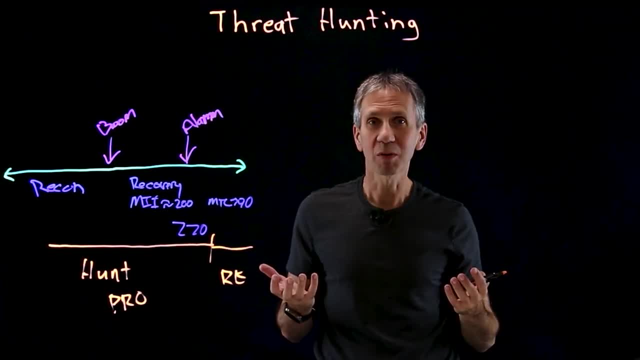 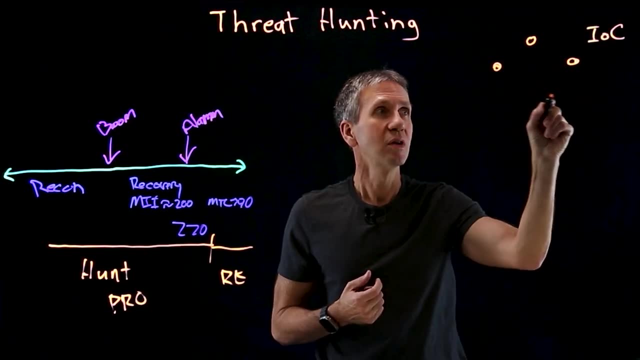 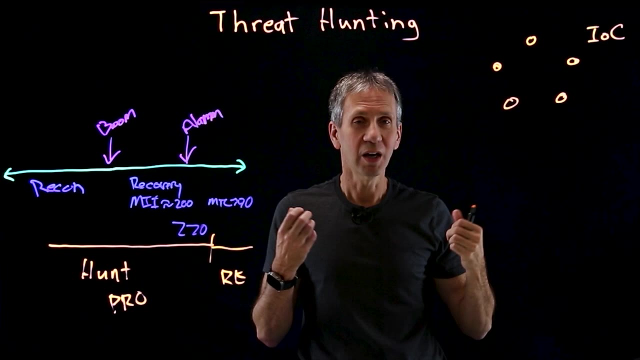 really happened yet or are in the process of happening, So no alarms have gone off. What are we going to use? Well, we're going to use things like indicators of compromise. That's information that we can gather from our systems that tell us that someone has done something here, that 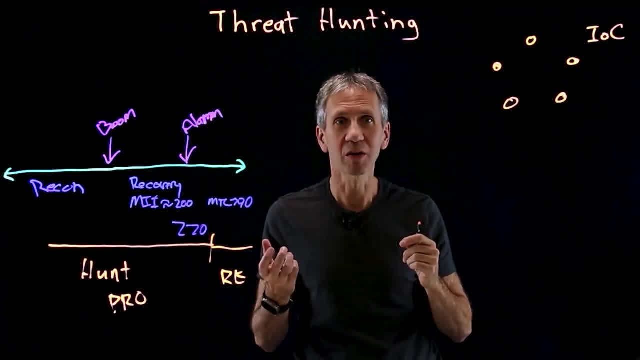 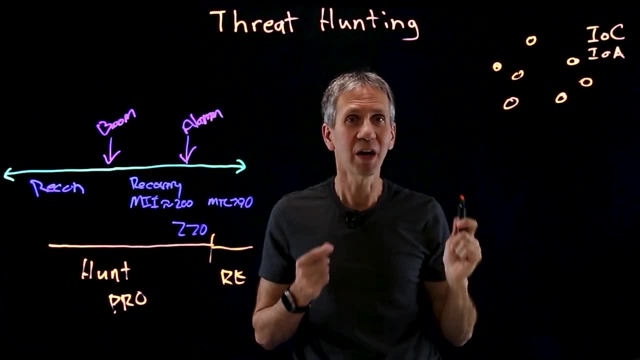 has breached. Maybe it's a small hole here, a small hole there. There are other things like indicators of attack that may be in here as well. It says someone is knocking on the door. They might not have fully gotten in, but they might have gotten in. So we're going to take that information and we're going to go back. 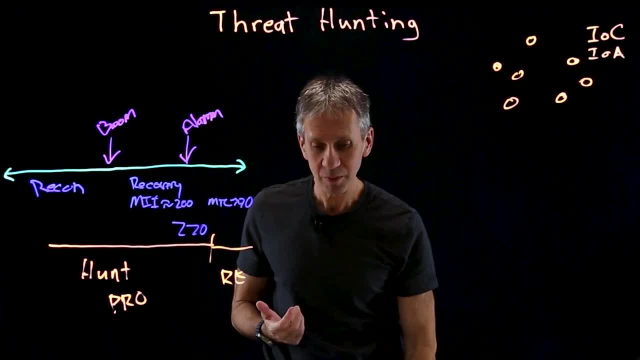 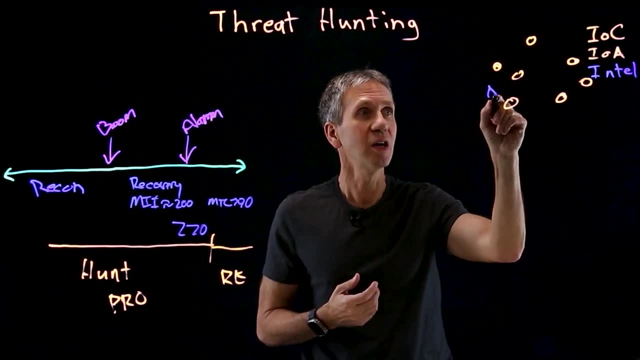 and look at it, You can see that they did some things that we should be concerned about. Other sources of information would be security intelligence threat feeds, so intel feeds that tell us that there are certain types of vulnerabilities that are being exploited on the. 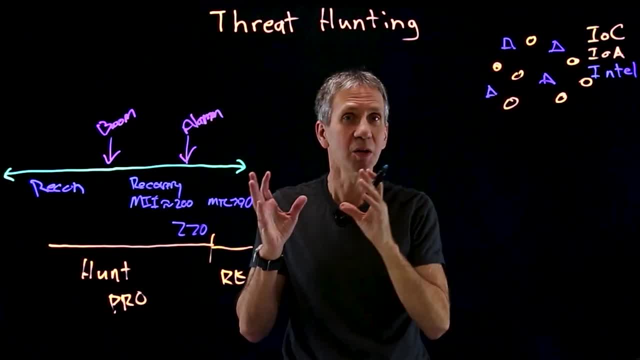 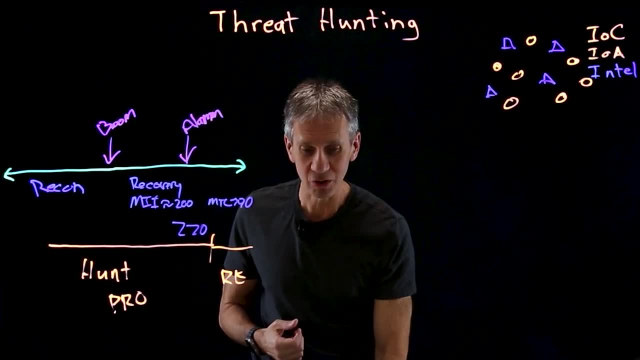 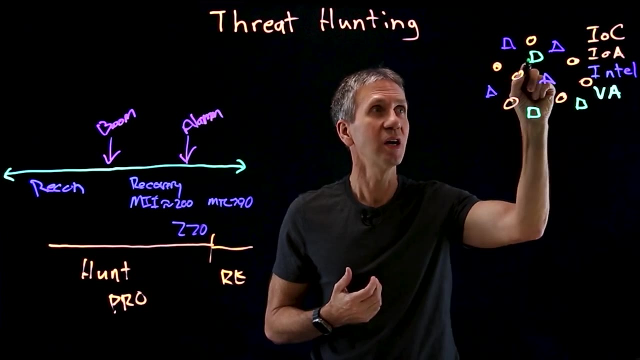 internet these days and certain things that are happening, maybe in a particular sector or in a particular geography. This is security intelligence. We'd like to use that kind of information and leverage it to our best ability as well. Speaker 1 could do some vulnerability scans on our environment And that would tell us what the bad 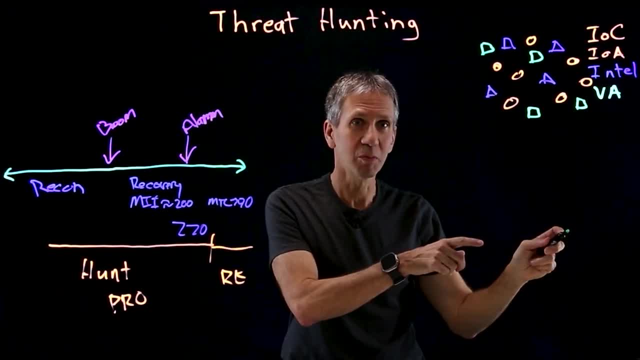 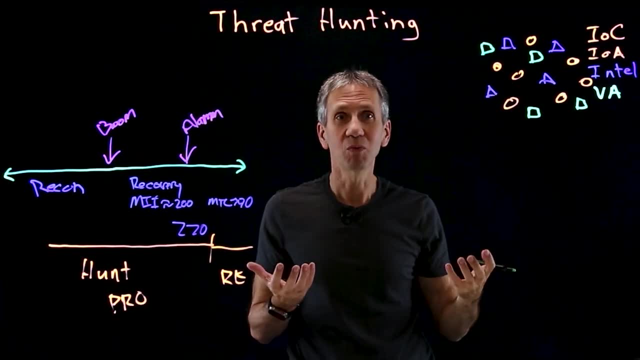 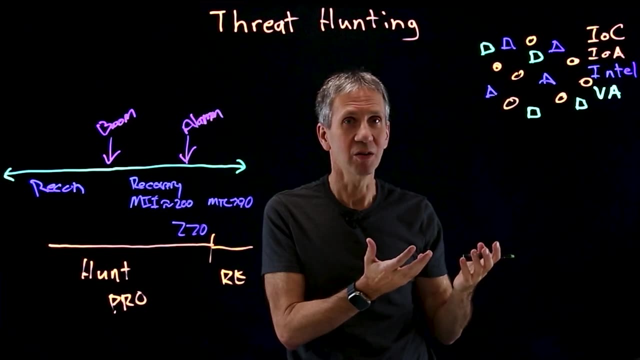 guy is also seeing, And that is that there are vulnerabilities here, There are systems that are weak here. This is the soft underbelly. This is what the bad guy is doing. Why wouldn't we do the same thing Then? an intelligent threat hunter who has some experience and some insight into this? 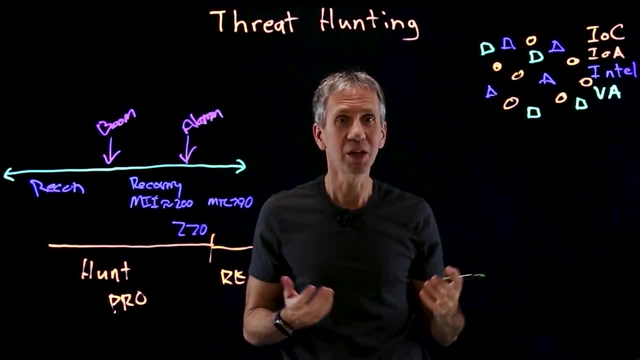 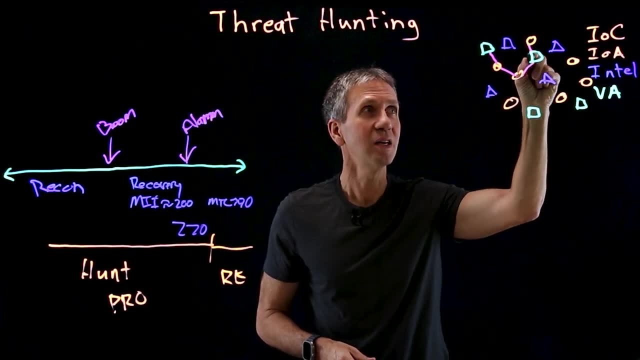 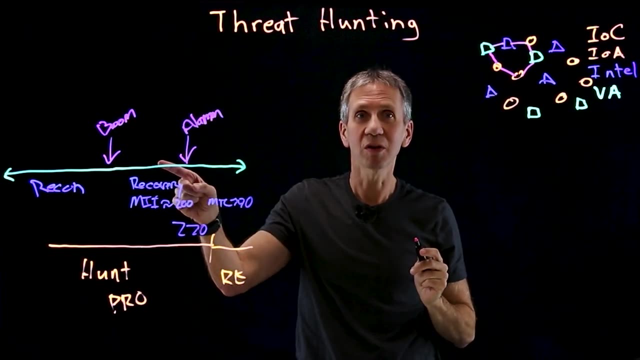 is going to use basically their experience and a little bit of intuition to connect the dots And say: these things that seemed isolated in fact are not. They're all grouped together. We connect the dots and we realize, before the boom has occurred, that in fact this is the setup. 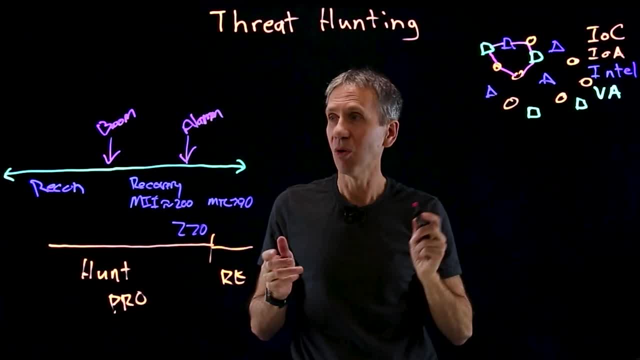 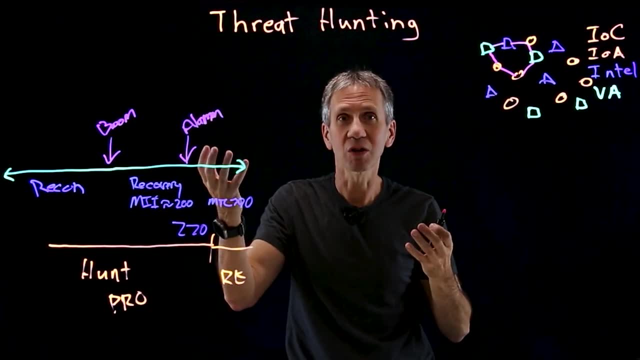 that's about to result in a data breach, Or it could be in this range of time, when some things maybe have. we've already been attacked, but the alarm hasn't gone off. But we're going to see the telltale signs And those are the things that we're looking for. 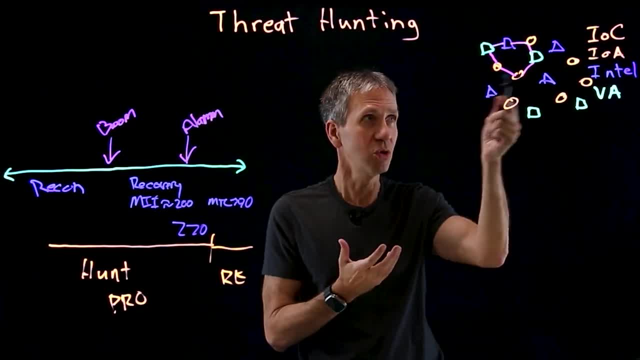 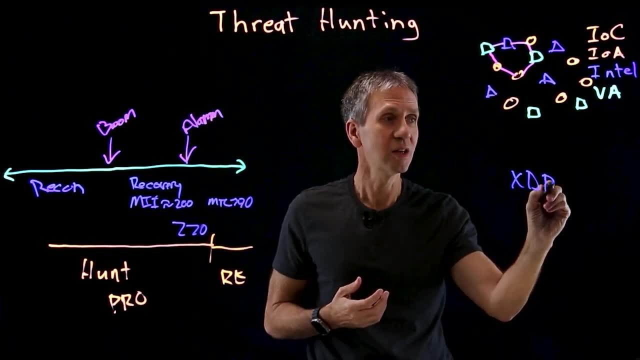 Now, what would an experienced threat hunter use in terms of the tools to gather all of this information? Well, they would use some tools like an XDR extended detection and response capability, And I've talked about this in a previous video. Another thing they would use: 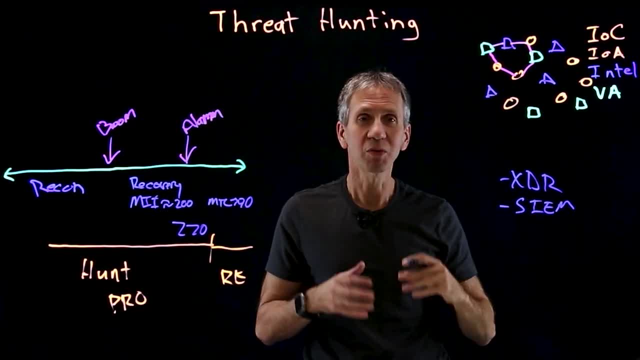 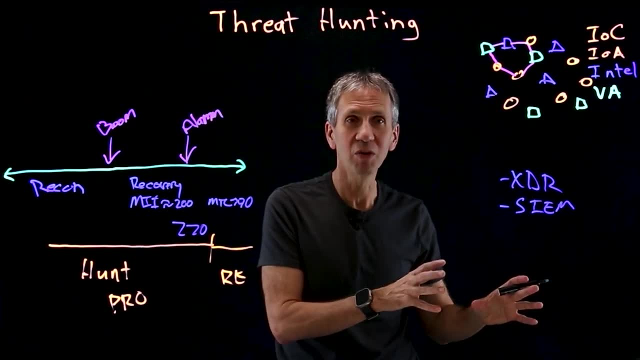 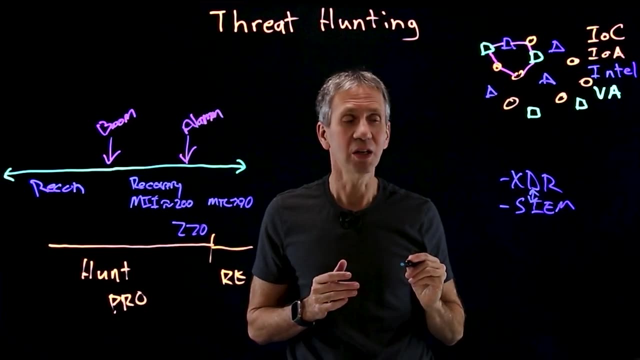 is a security information and event management system, Something that goes out and gathers information from all of my sources of security: telemetry, all of the logs, all of the flow data, all of the different sources that might give me and all of the data that I need to get the information. So that would be the security. 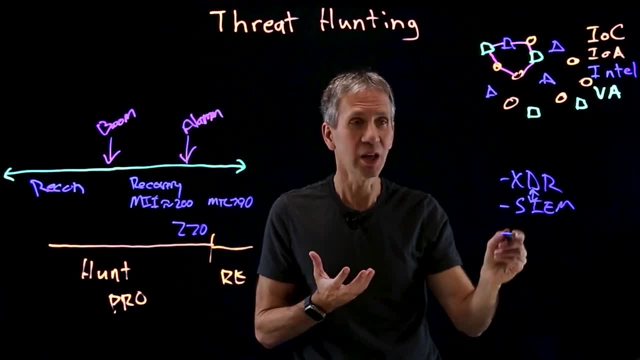 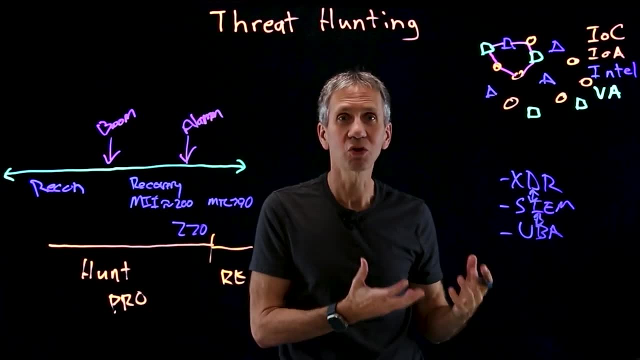 intelligence, And these two, in fact, can be related in feeding to each other. And then another related technology that often relates to these as well is a user behavior analytics capability, And the UVA would look for anomalous user activities. Here's a user that's performing. 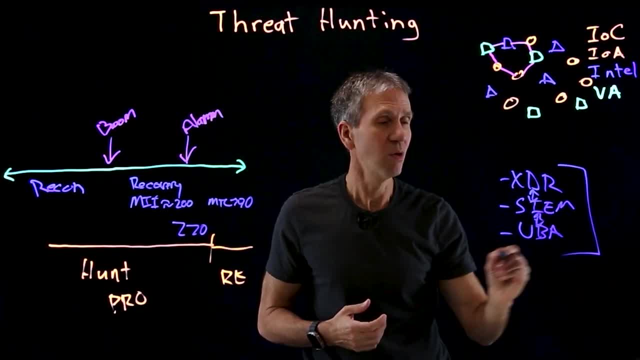 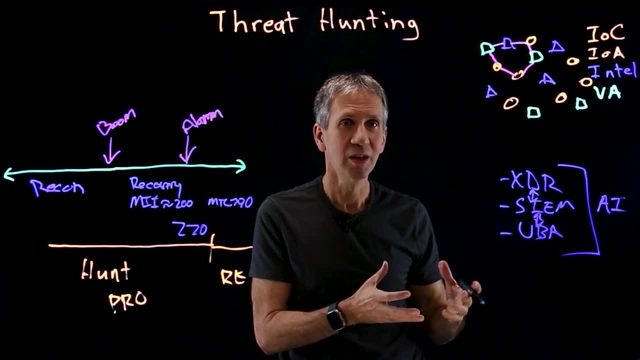 differently than what their peer group is doing and therefore they're drawing suspicion. And then we would ultimately want to take all of those technologies and infuse them with artificial intelligence so that we can't do that, can get to the point, find the source, get to our investigation faster and do the reporting and 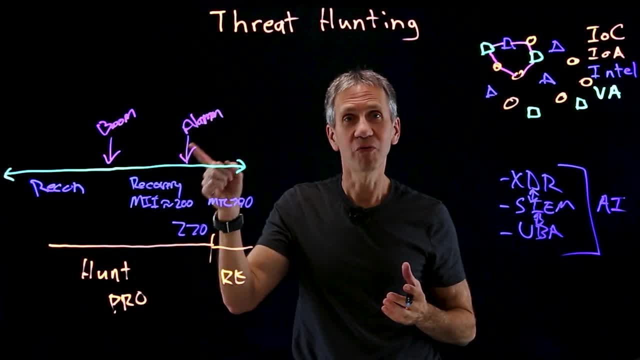 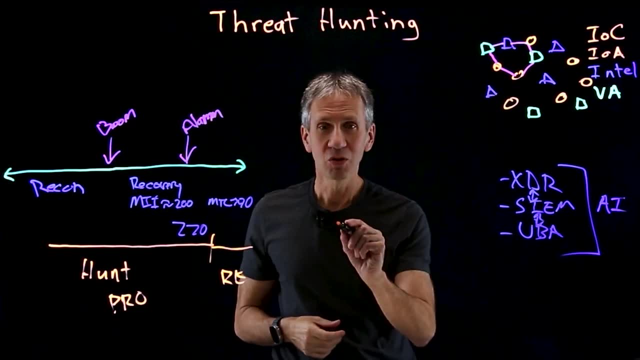 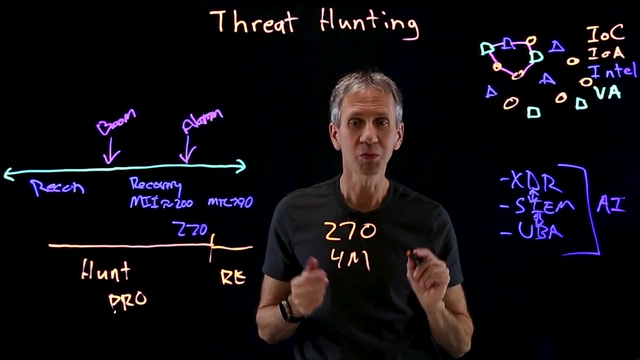 hopefully uncover this issue before the boom and if not at least very soon after the boom, because what we're trying to do is avoid two numbers. there's one number, 270, and another number, four million. what do those mean? 270 is roughly the number of days between boom and containment.